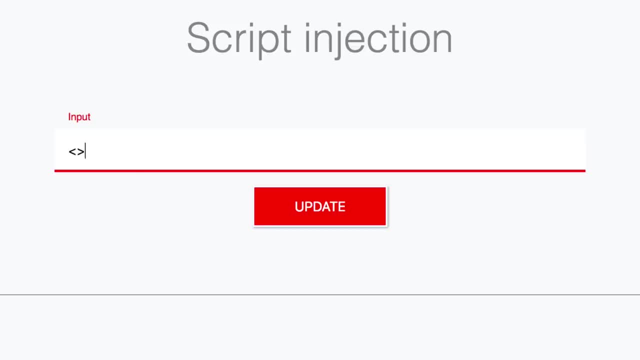 HTML tag using less than and greater than characters surrounding an element name, like P for paragraph. Then add some content and then add a closing tag after that, which is just the same as an opening tag, only there's a slash in front of the element name. Then click the update button. 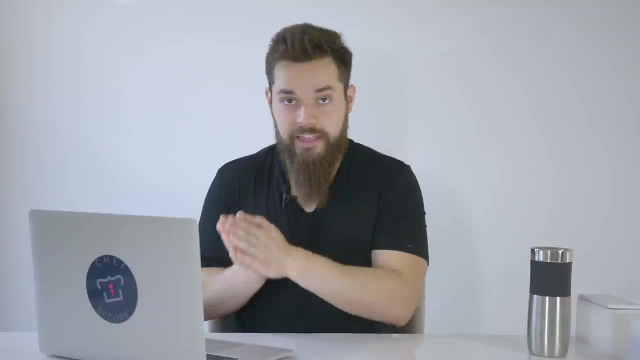 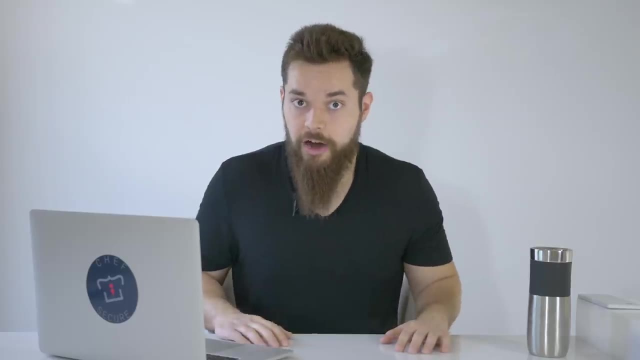 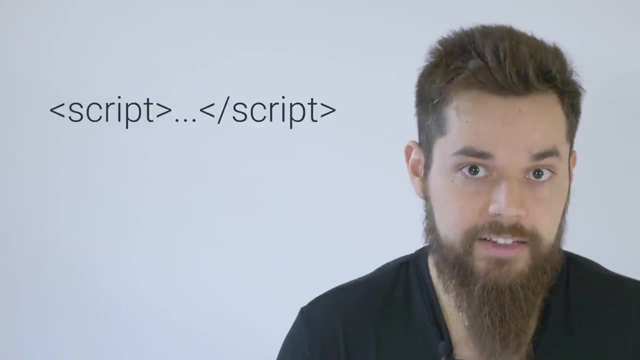 You see that, instead of writing text, you actually change the HTML of the web page by adding a new paragraph element. While simple, this is very, very powerful, because JavaScript controls the web page And if you can inject a script element instead, you now control exactly what happens in the browser. And this is how XSS works. So go ahead and 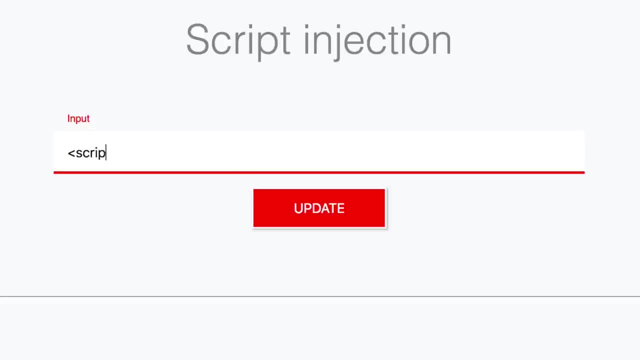 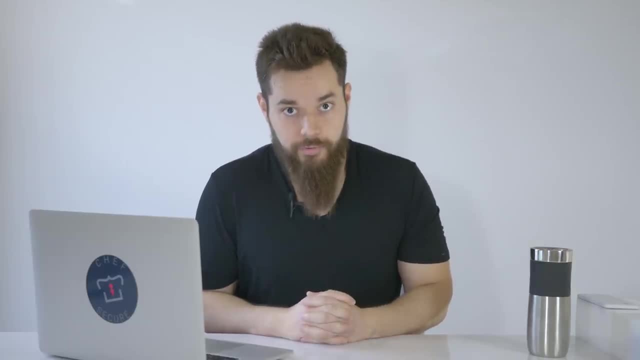 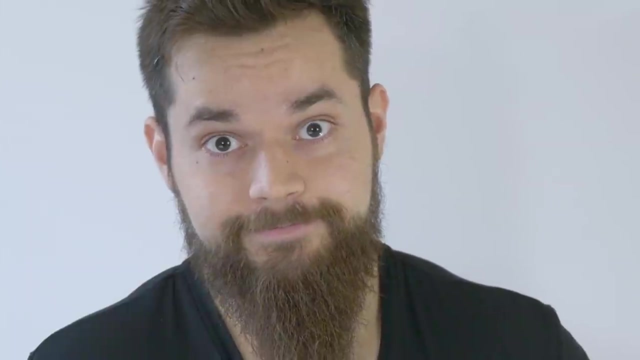 inject script tags. this time Start with your opening script tag, followed by your closing script tag. Now for the content that goes inside. This, my friends, is where we enter the f***ed up world of JavaScript, Wonderful world of JavaScript. JavaScript can be confusing at times, but what it? 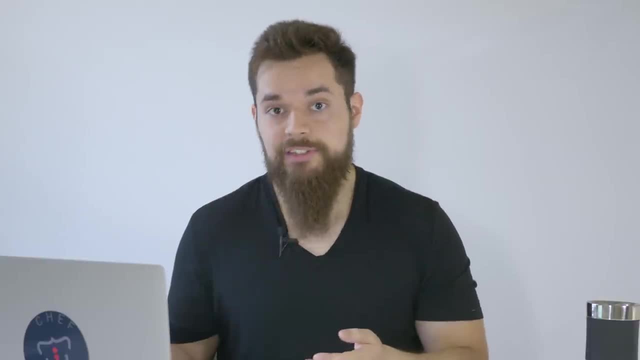 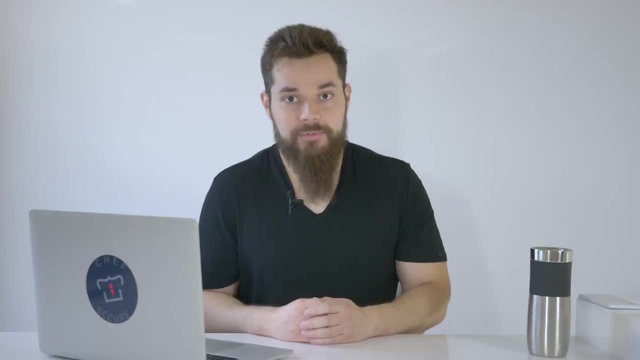 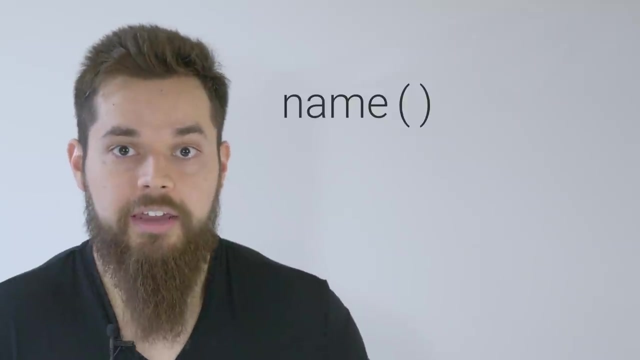 does well. it does exceptionally well, like letting you hack websites or making them more interactive. Performing actions in JavaScript is like any other programming language, where you just call functions. You can do this by typing the name, followed by parentheses And anything that goes. 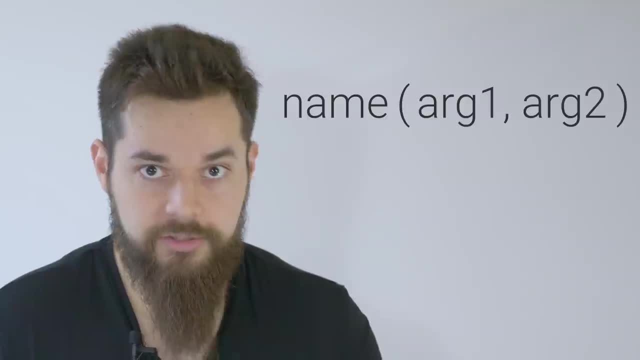 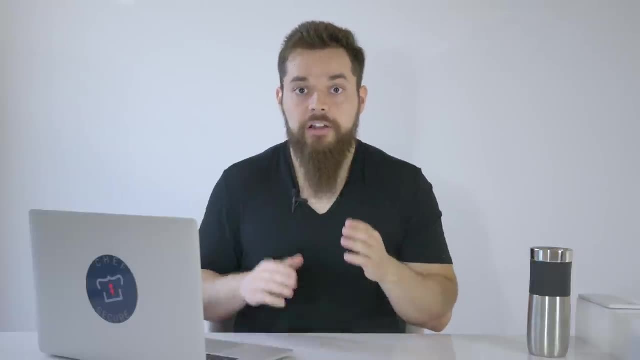 inside the parentheses, gets passed as data or arguments that the function can use And, like other programming languages, you can set values using an equal sign. Right now, try calling the alert function within your script tags, So type in alert followed by parentheses. 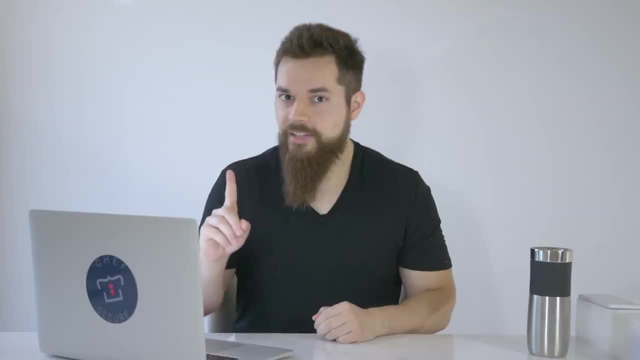 Then click the update button and watch your script execute, Because you see this alert pop up. it means your script was injected into the page successfully and ran due to an XSS vulnerability. While you're at it, get some practice with arguments as well. 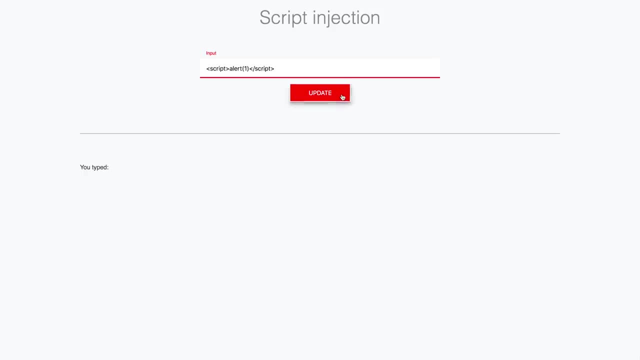 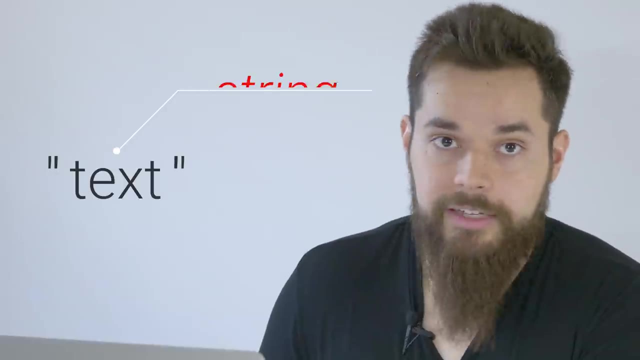 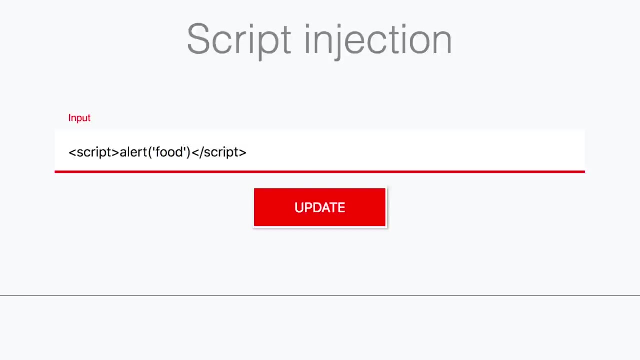 So type in the number one to the alert function, click the update button and you'll see it. alert one, Or pass in text surrounded by either single or double quotes to make a string and you can alert something you really love. I'm going to alert food Because I love food. I'm all. 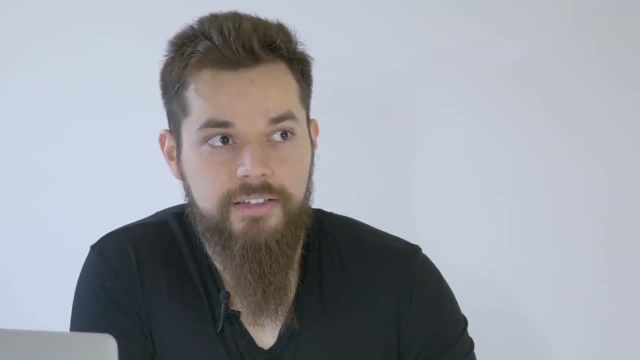 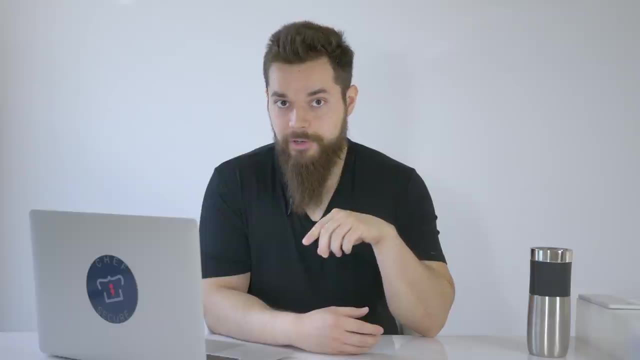 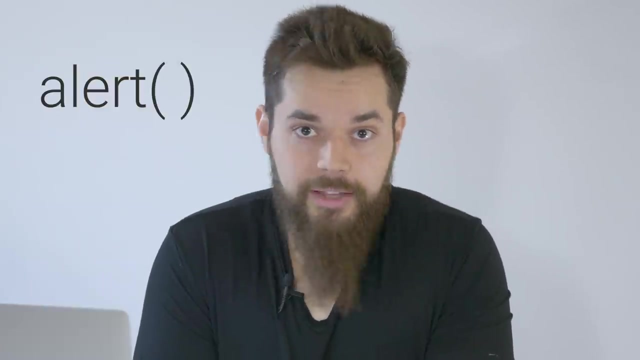 always thinking about Wait a second Chef. secure Alerting is the most common function used by both cyber criminals and security researchers alike to find vulnerabilities in websites. Now, keep in mind that the alert function is just a placeholder, showing that a script can be injected And once a vulnerability is found. 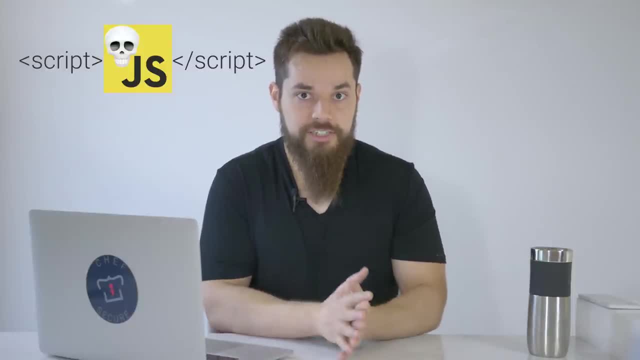 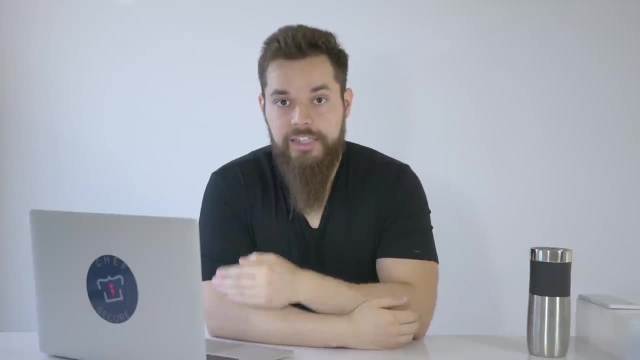 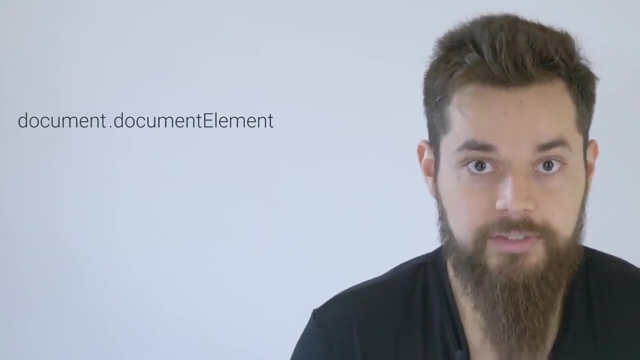 an attacker can easily replace this with a malicious exploit that causes much more damage. Consider something similar simple. Instead of alerting in our example, let's just destroy the whole web page by removing all the HTML In JavaScript. documentdocumentElementinnerHTML contains all the HTML of the web page, So 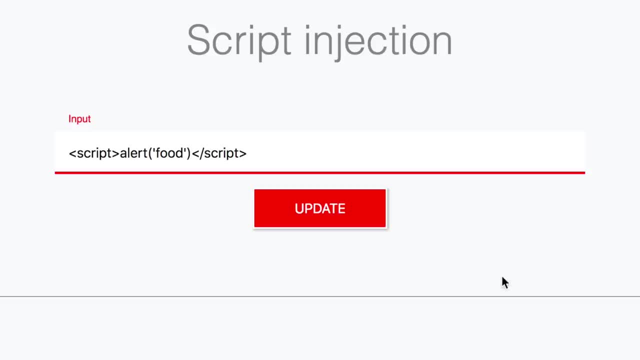 just change it by setting it equal to an empty string. In our example, if we type that in documentdocumentElementinnerHTML equals empty string, click the update button and it's gone. I'm going to show you more about how cybercriminals can exploit websites in a later. 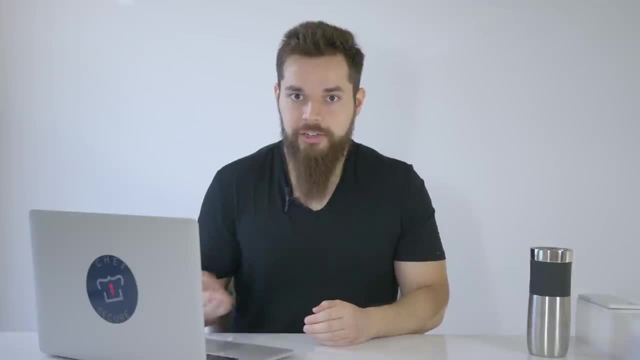 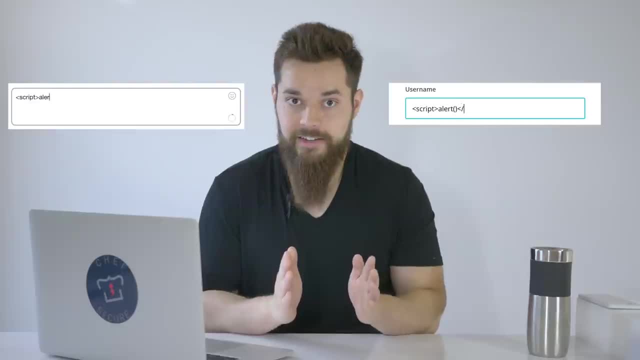 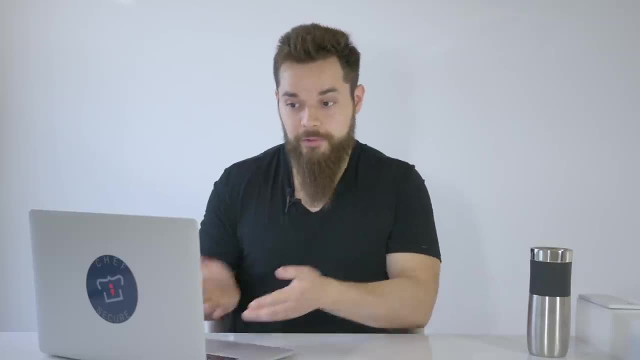 username or a status update. There's always a chance that it could contain an XSS vulnerability, so it's worth a shot. Of course, websites do have protections against XSS, Some of them even built directly into the frameworks on which they're built. But despite this, 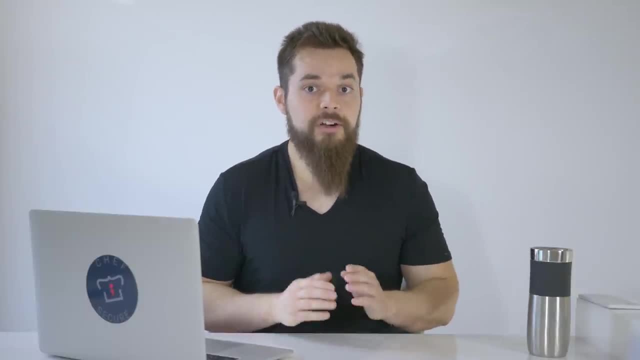 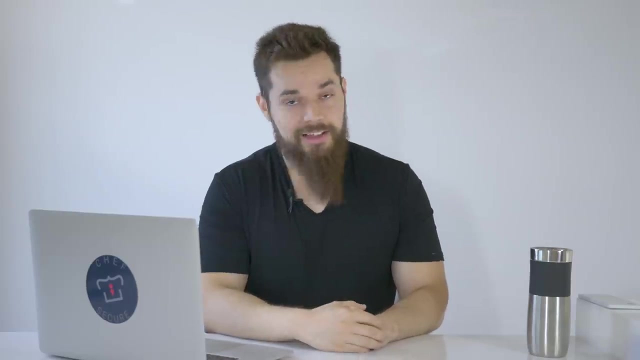 and despite the frameworks being around for several years, the number of XSS vulnerabilities is still rising like crazy, And that's because writing secure, resilient code can be quite tricky at times, And even with automatic protection, you can still screw things up pretty badly. Trust me, I've done it more than once And I'll do it again. I promise. 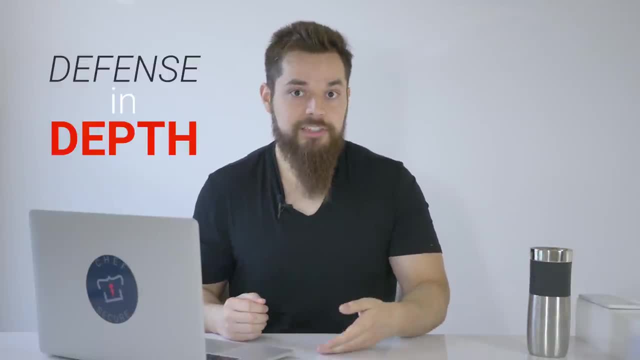 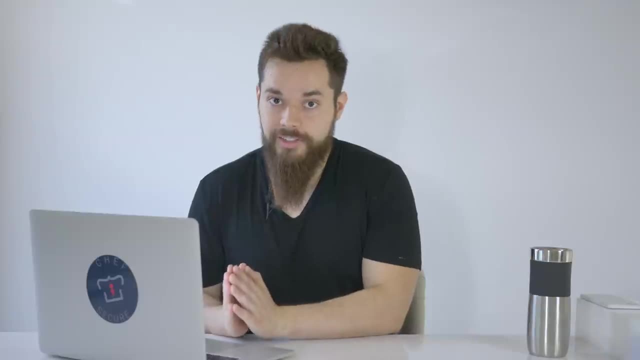 But that's the point of having defense in depth, which I will teach you as we go along in this course. But mistakes happen, so let's look on the bright side. At least there are plenty of vulnerabilities to find and fix before cybercriminals can come and hack your application. 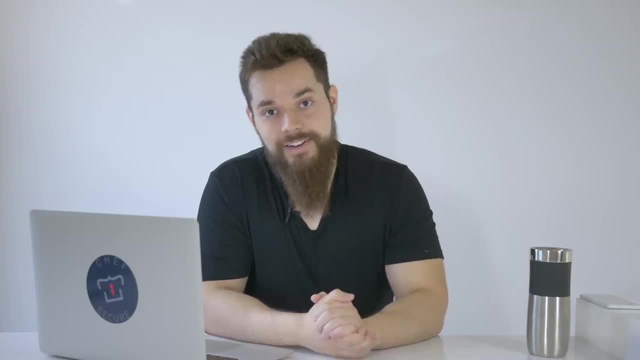 Wait. that's not comforting at all, But that's all the time I have for now. Goodbye friends. 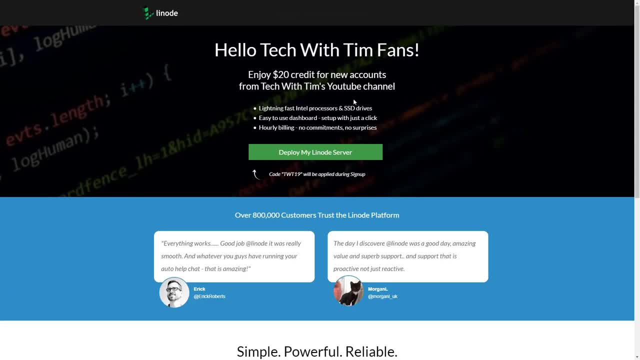 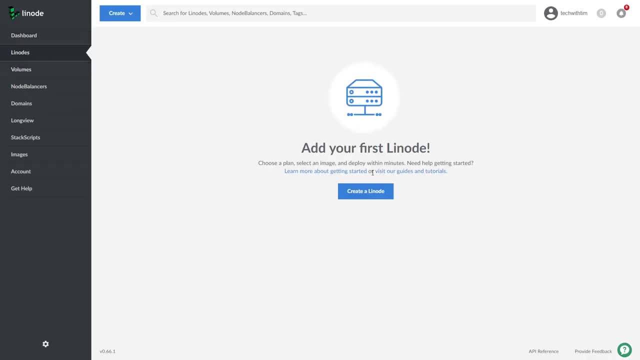 Before we get started, I need to give a massive thank you to Linode for sponsoring this video. They make it easy and affordable to host your site or service in the cloud, offering no-nonsense hosting with plans starting at just $5.. This means no surprise fees or overages, like you might. 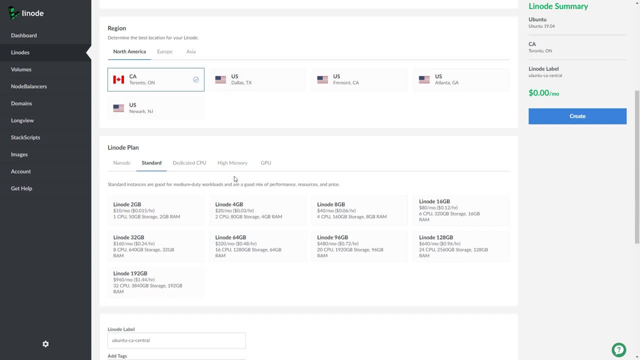 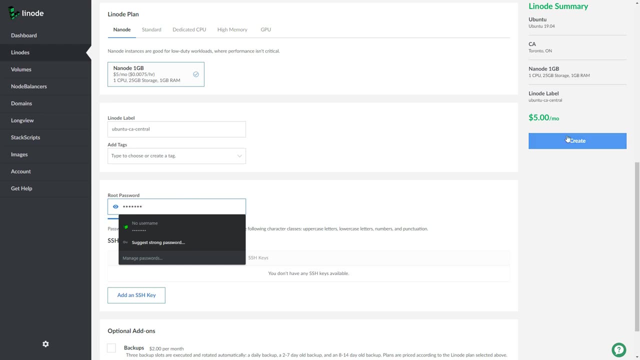 have gotten from some more entry-level hosting companies. Now Linode also has a full API that works with tools like Terraform and Kubernetes, making it an awesome environment for development projects. Maybe you've used an entry-level hosting service before. Well, Linode is your step up to. 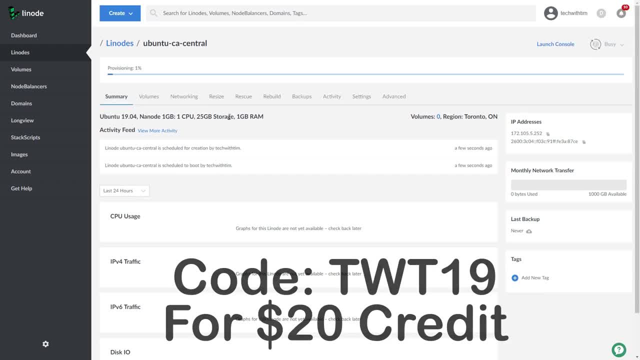 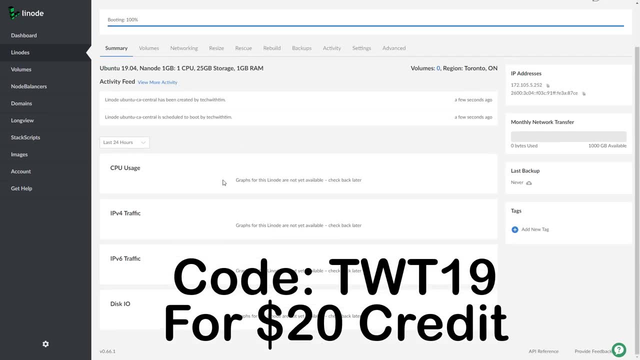 powerful, fast and fully configurable cloud computing. Anyways, go ahead and sign up with the link below and take advantage of a free $20 credit using the code TWT19.. All right, so let's talk about binary search trees Now, before we get into the search tree, 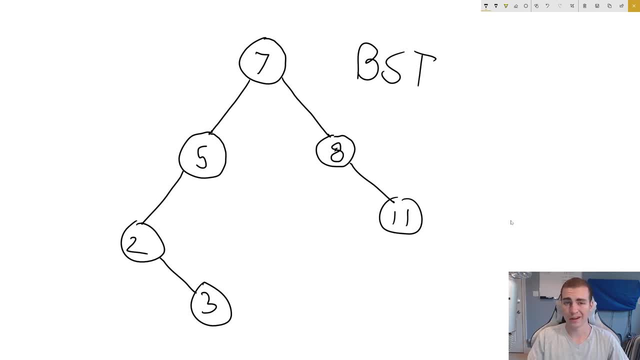 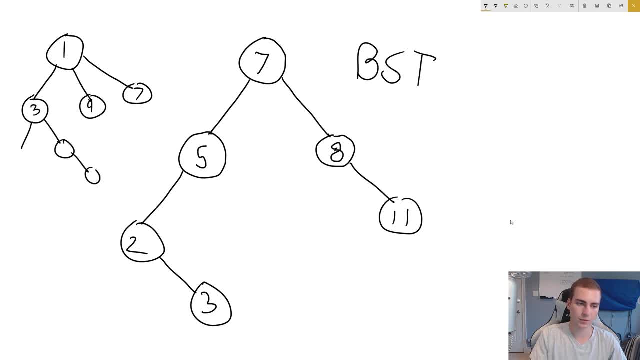 branches. maybe these ones have a few branches coming off, maybe this one has one, and it keeps going right, And that's what a tree is. Now, a binary tree is really basically just a tree that only has at most two branches for every node. Now what that means is each.